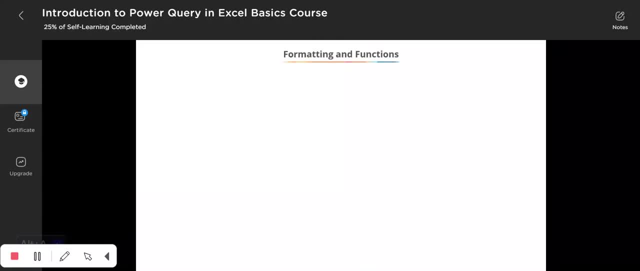 Formatting and Important Functions. In this lesson we will learn about custom formatting, how to use it and implement logical, statistical and mathematical functions. Let's say we need to differentiate the sales value from a given dataset as above target, below target and met target. As a dataset can be huge and complex. 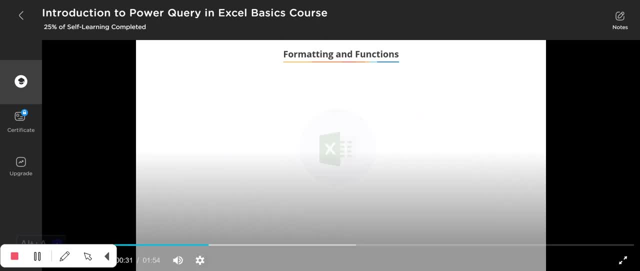 differentiating each value manually would consume a lot of effort and time. Here we can use Excel features such as formatting and conditional formatting, which will enable us to perform this task easily. Formatting, as the name suggests, helps us format the data using different 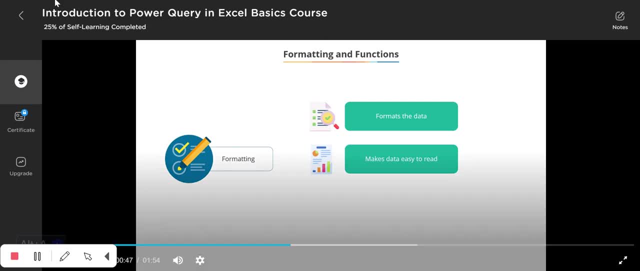 techniques making the data easy to read in the required format and analyze them. The right formatting technique applied to the worksheets can help users present the data efficiently. Conditional formatting helps us to visually explore and analyze data, detect critical issues and identify patterns and trends. Conditional formatting helps to add patterns and trends to. 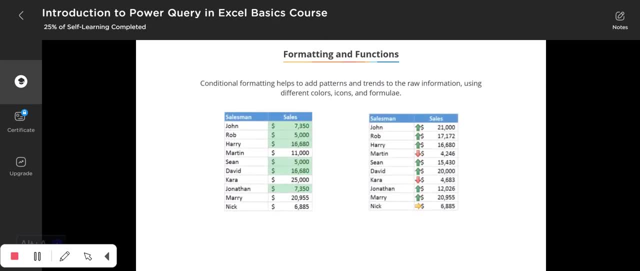 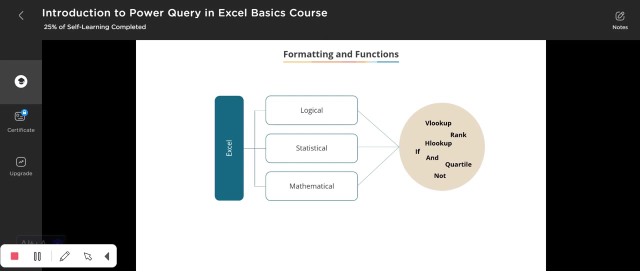 the raw information using different colors, icons, formulas, etc. Sometimes we also need to perform mathematical operations and calculations within our dataset. In such cases, Excel provides a large number of logical, statistical and mathematical functions, such as VLOOKUP, HLOOKUP, IF NOT, RANK QUARTILE, and many more that can help the users to perform. 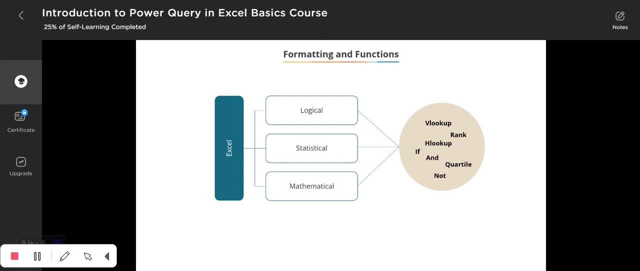 calculations ranging from basic to complex operations. These inbuilt functions help us manage data and perform descriptive statistical analysis. Excel also offers a wide range of important formulas that help perform many common tasks. These formulas may be as simple as basic addition or could be a complex combination of inbuilt Excel functions. Before going into details, 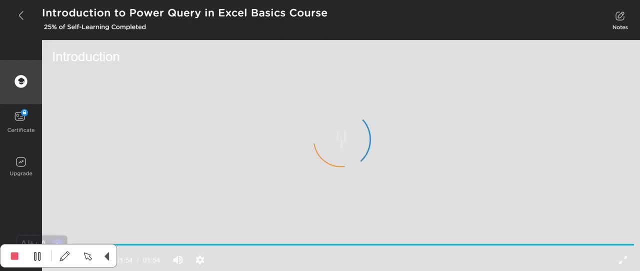 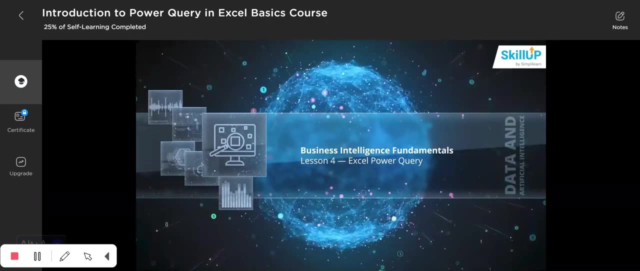 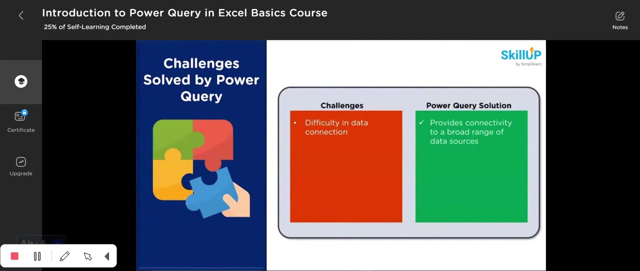 let us start this lesson by defining the formula. Now let's look at the challenges solved by Power Query. Earlier in Excel, there was difficulty in data connections. Now, using Power Query, you can connect to a broad range of data sources, such as relational databases, web files. text. 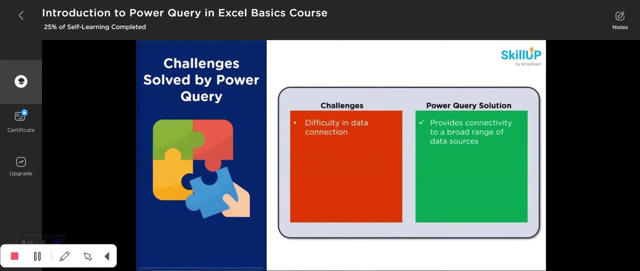 CSV, JSON files and even fetched data in the cloud. Volume, variety and velocity are the characteristics that define big data. It was a major problem to handle such data. Now, Power Query enables you to transform your data into a large number of different types of data. 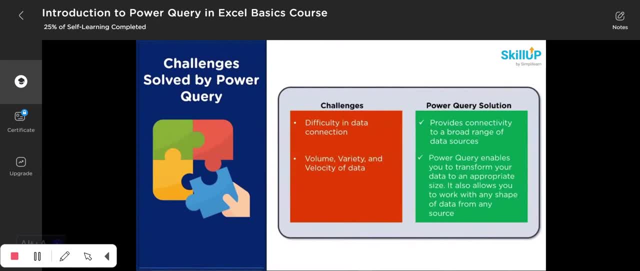 It also allows you to work on any shape of data from any source. Earlier, updating your data and refreshing it in real-time was an issue. Using Power Query, a repeatable process query is adopted to update the data in real-time and in the future. In Excel, it was not so easy to reshape, transform and manipulate data, But 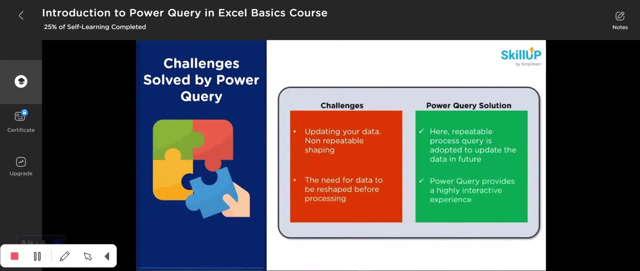 using Power Query provides a highly interactive experience and sophisticated tools to prepare your data. Now, from Excel 2016 onwards, Power Query on Windows has been fully integrated into Excel. Now, Power Query has been fully integrated into Excel. Now, Power Query has been fully integrated. 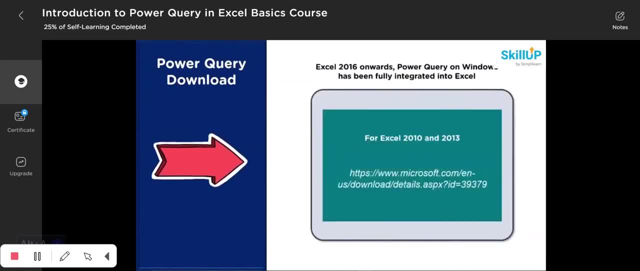 into Excel. But in Excel 2010 and 2013 for Windows, Power Query is a free add-in. You can go ahead and download the link. Once installed, the Power Query tab will be visible in the Excel ribbon. Now coming to the features of Power Query. So Excel Power Query allows you to clean. 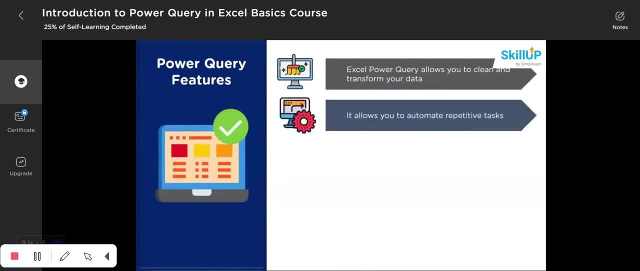 transform, manipulate and process your data for analysis. It helps you to automate repetitive tasks that you want to do it over and over again. You can search for data sources and make connections as and when you want. Power Query helps you to prepare and shape the data in the 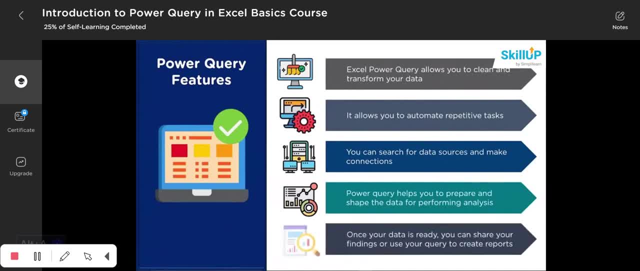 right format for performing analysis. And finally, once your data is ready, you can search for data sources and make connections as and when you want. And finally, once your data is ready, you can search for data sources and make connections as and when you want. And finally, once your 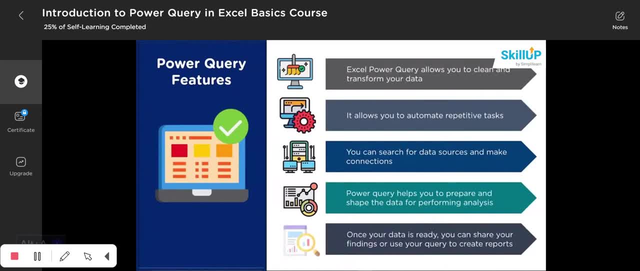 data is ready. you can search for data sources and make connections as and when you want. You can share your findings or use your query to create interactive reports and dashboards. Now let's have a glance at the demo that we are going to work on in this video. So we'll look at how to 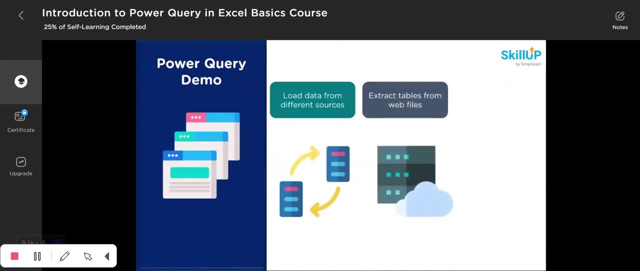 load data from different sources. You will understand how to extract tables from web files, So we'll extract tables present on Wikipedia pages. Then you'll learn how to sort and filter data. Up next, you'll see how to group your data, how to split a column into multiple columns. 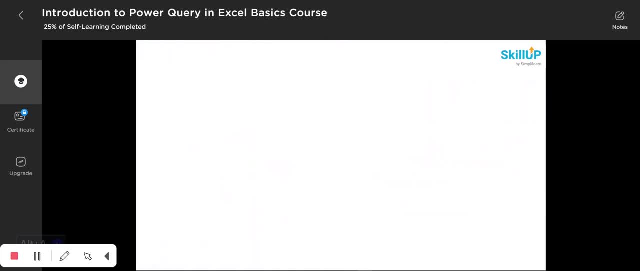 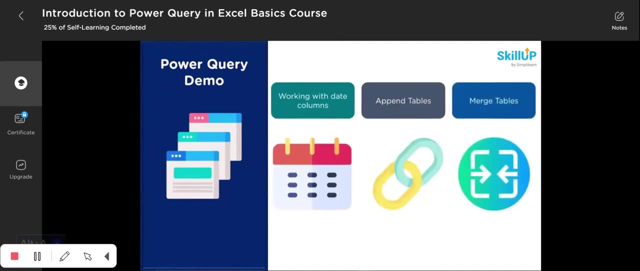 and then pivot and un-pivot your table. Then you're going to work on date columns and make some transformations, Understand how to append tables and merge tables vertically and horizontally. Now let's open MS Excel and start with importing a simple 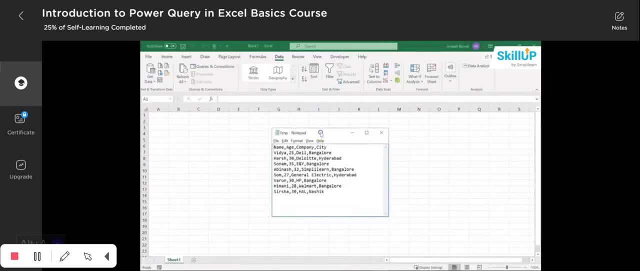 text file. So you can see here I have my Excel file opened And in the middle you can see I have my employeetxt file. Now, this is a comma-separated file, meaning that the values are separated by commas. as you can see it here, The columns have been separated by commas. 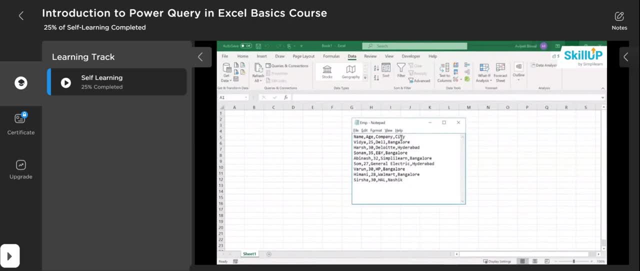 See how easily you can import this data from your data. Now let's open MS Excel and start with importing a simple text file. Here I'm using Excel 365 or Office 365, where Power Query on Windows has been fully integrated into this version of Excel. So what I'll do is: first let's go to the 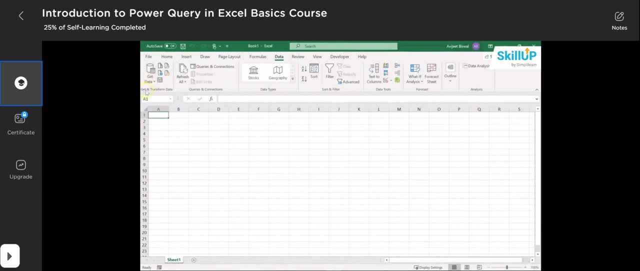 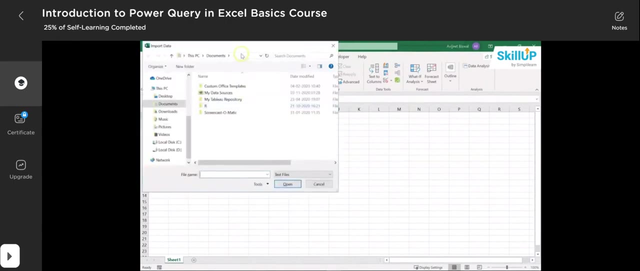 data tab And you have this section called Get and Transform Data. So I'll click on Get Data. Under Get Data I'll go to From File and select From Text, Slash, CSV. Once I click on it it will ask me to give the location where the file is there. So my file is. 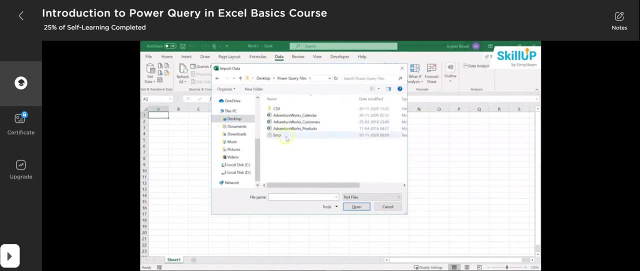 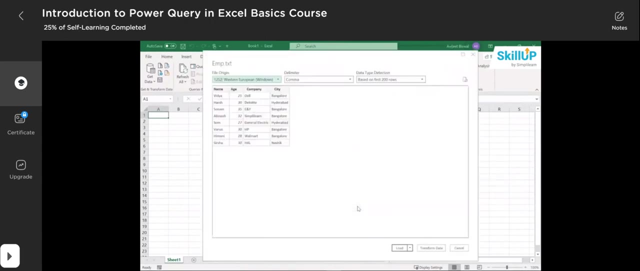 on desktop. I'll click on Power Query Files And here you can see I have my employeetxt file. You can see the type here. It says X document. Click on EMP and hit Import. Now this will take some time to import the file onto Excel. It's establishing a connection. you can see There. 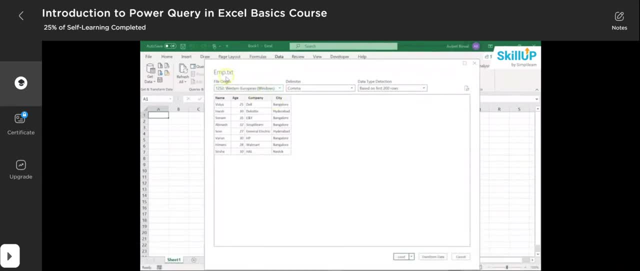 you go. So here you can see the file name: emptxt. You can see the file origin. As I said, the delimiter is comma And we have the data type detection. And here you can see we have our text file. So Excel Power Query feature has automatically detected the. 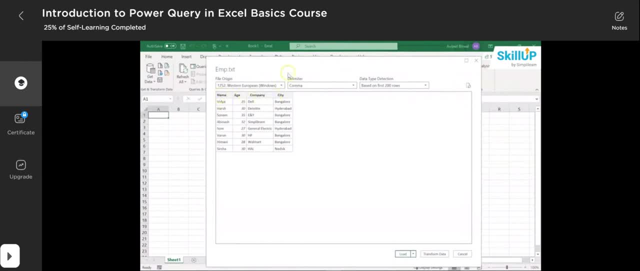 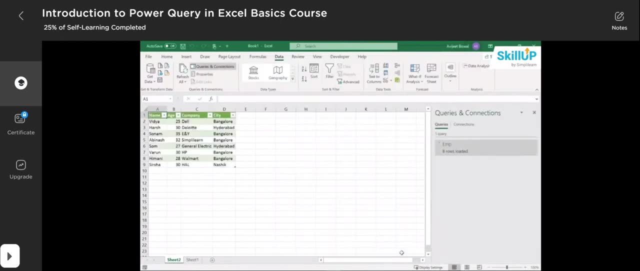 column names. So we have name, age, company and city as our columns And these are the values. Now let's hit Load, So this will load all the rows and the columns onto Excel. There you go. It was really quick. Excel has automatically loaded our text file, So we 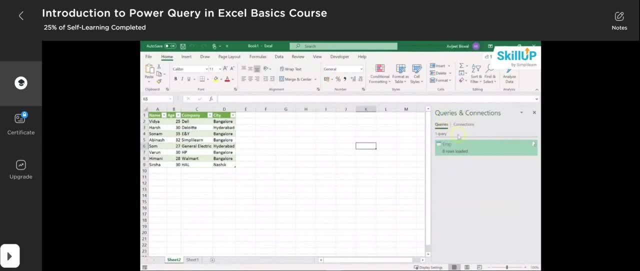 can see here. we have another tab called Queries and Connections. So we have made one query and have loaded the employee data. It gives a preview also. You can see it here And if needed later you can go to Edit and change some values That we'll see later. Now you 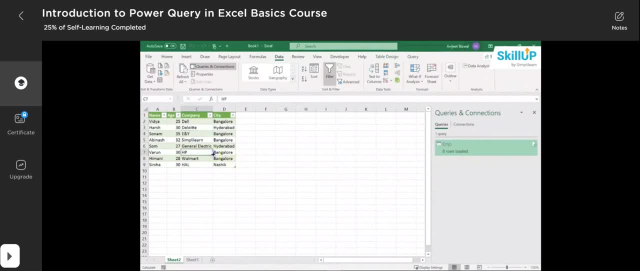 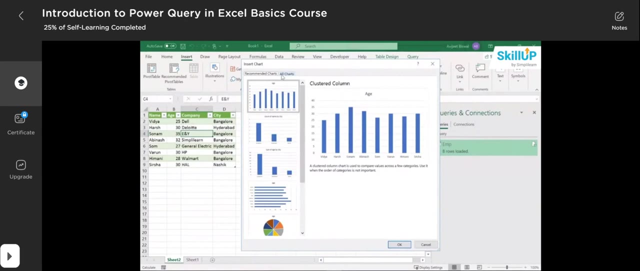 can use this data to create simple visualizations, So let me show you how to do it. So let's first select the data and we'll go to the Insert tab. Under Insert tab, I'll click on it. I want to know how many employees belong to a particular city, So I'll click on the. 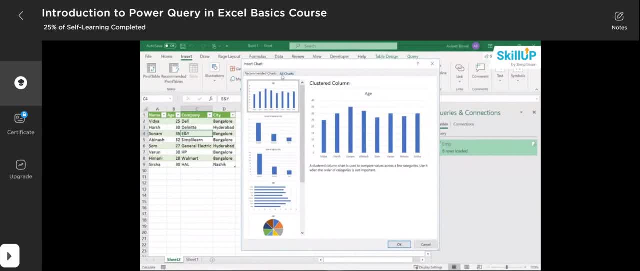 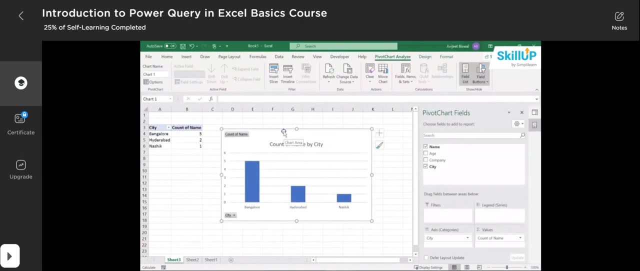 second chart which says the count of name by city, And I'll click on OK. Here you can see we have a nice clustered bar chart And you can see in Bangalore there were 5 employees, In Hyderabad we had 2. And in Nasik we had 1.. You can see the count here. This is a pivot. 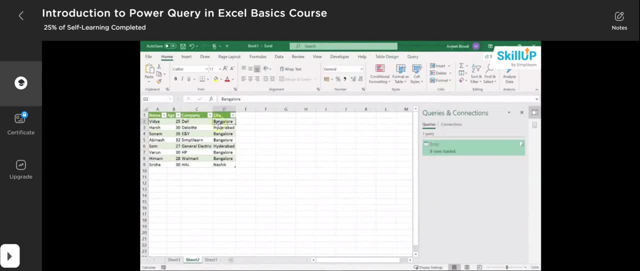 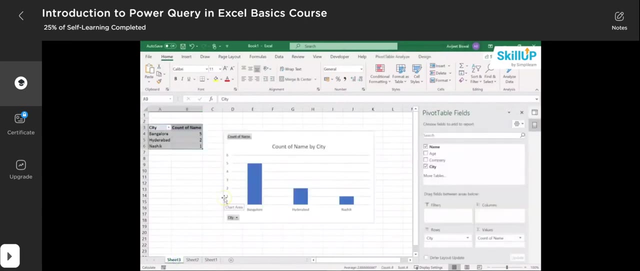 table. If you go back to our actual data here, you can see in Bangalore we had Vidya, Sonam, Avinash, Varun and Himani, And there were 2 more people from Hyderabad and 1 from Nasik. So you can use the Excel Power Query feature. 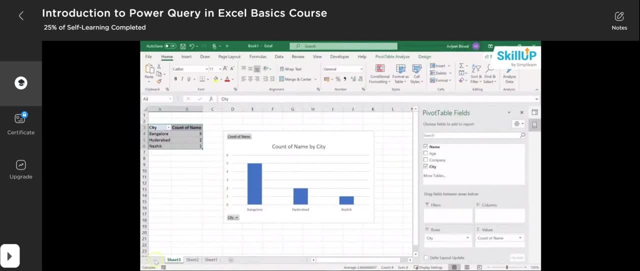 to import data onto Excel and make some visualizations. Now, if you want to fetch some data that is present on the web or on the internet, Excel Power Query features and functionalities can help you import those data as well. We will now see how to import data from the web. 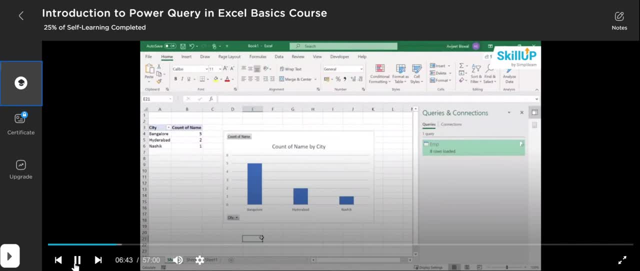 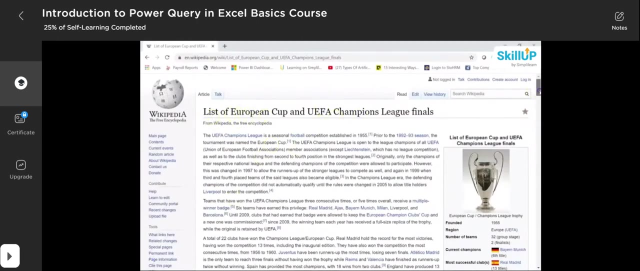 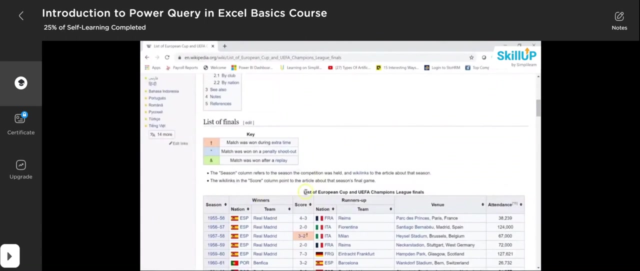 Here I'll be using a Wikipedia article on this page first. So this is my Wikipedia page on the list of European Cup and UEFA Champions League Finals. If I scroll down, you can see all the details here, And I would like to import this table which has the list. 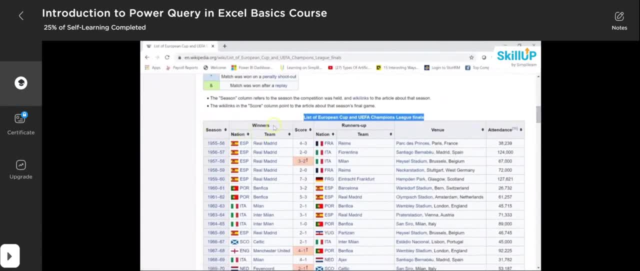 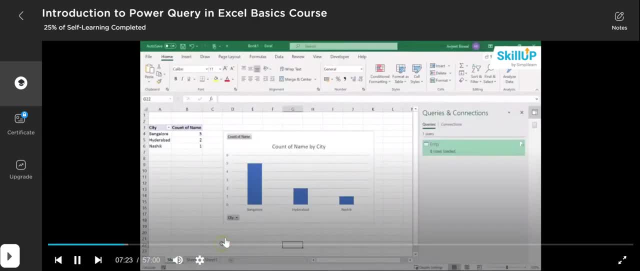 So we have columns like Season Winners- Scoreline and so on. So we have columns like Season Winners- Scoreline and so on. So we have columns like Season Winners. now let me open a new sheet. i'll go to sheet one and then on the data tab, under the get data, 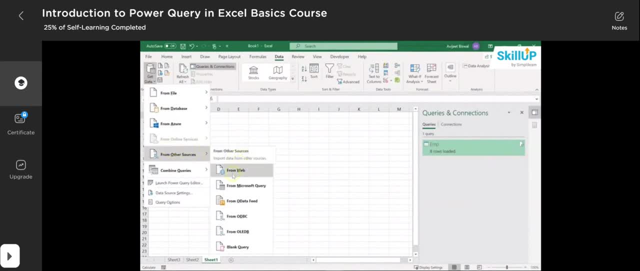 section i'll go to from other sources, and here i have from web, which allows me to import data from the web. either you can follow this path or, if you see, here there's an option to get data from the web. if i click on this, it is asking me to enter the url, so i'll paste the url of the. 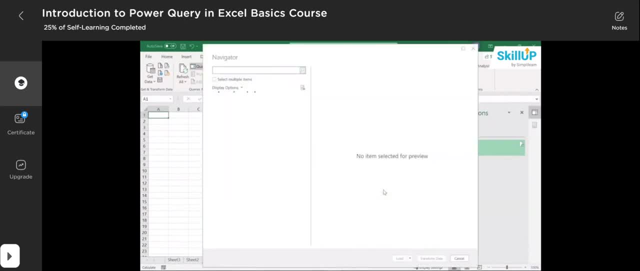 wikipedia page here and let's click on. ok, now it's navigating and ok, you can see. power query feature in excel has given us a list of tables which you can see. here we have something called document. there's a key table and here you can see there's one table which is extracted from the 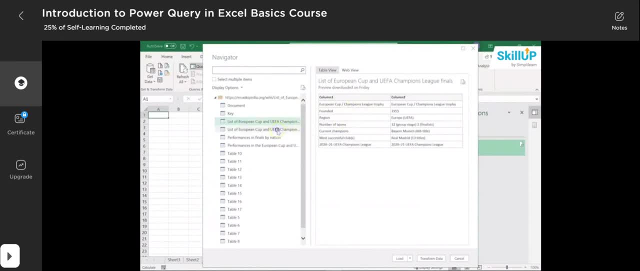 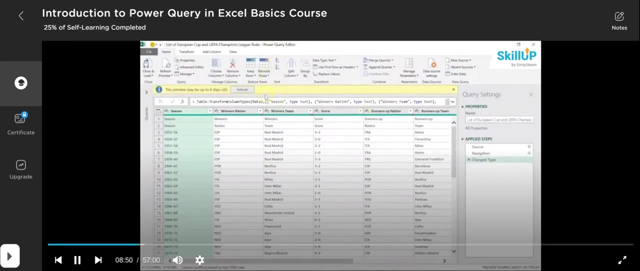 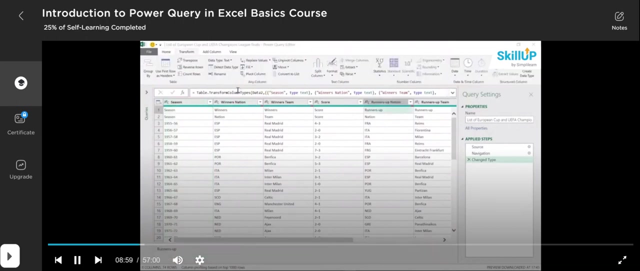 wikipedia page and the table which i am interested in is this table which has the list of european cup finals. you can see it here. excel power query feature has automatically detected these rows and it has given a list of call very editor. let me just click on refresh now. this is the most important section. using the power query editor, you can. 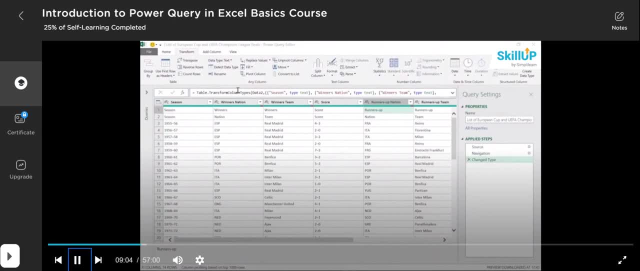 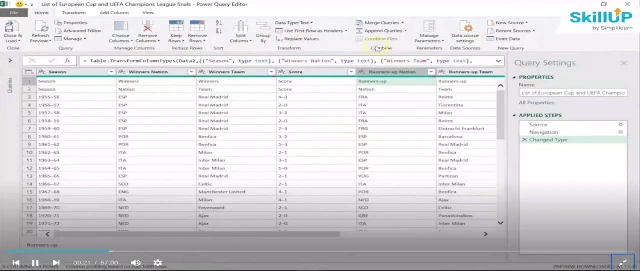 clean your data, filter your data, manipulate your data and make it ready for analysis. now let's explore a few tabs available here. so we have a home tab that has a query section. you can see. you can reduce rows, manage columns, sort the data, transform data, combine different tables. now there's another tab called transform, which allows you to select. 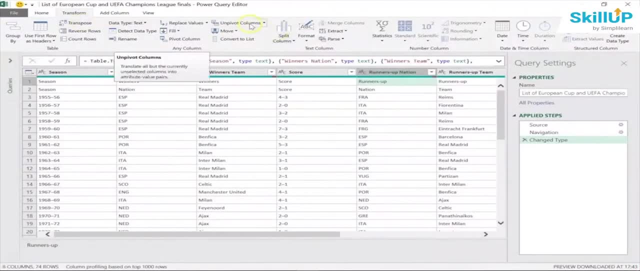 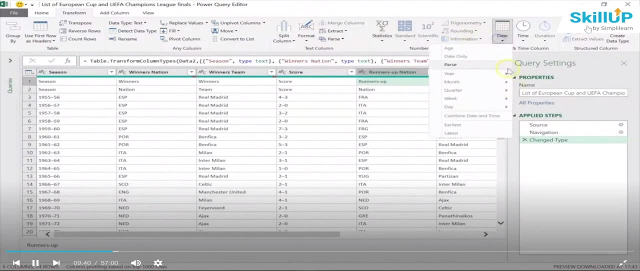 your data type, transpose your rows and columns. you go to pivot your columns and here you can see, you can find out some summary statistics and you can manage your date values as well. now, if you want to add some new columns to your data, you can do that as well, and you also 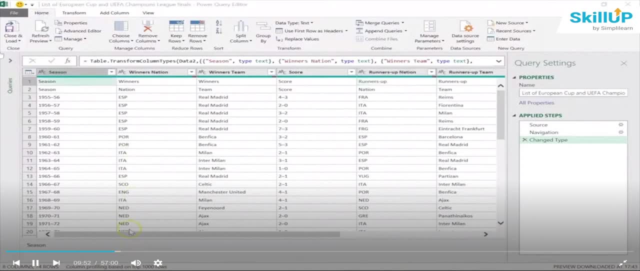 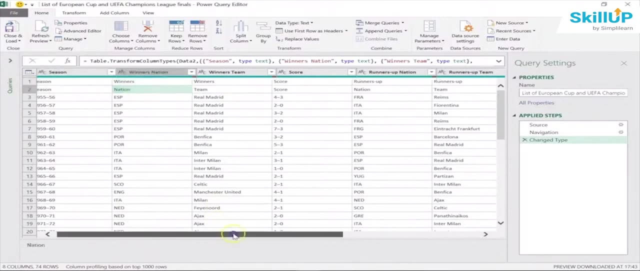 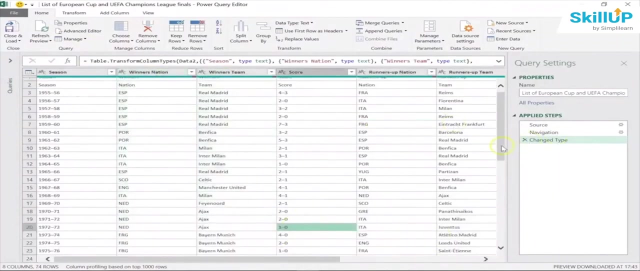 so have a view tab now here. if you see the first two rows, the values are the same. you can see season, season. these are all repeated, which you actually don't need, and these are pretty similar to our column names. similarly, if i scroll down, you see there are. 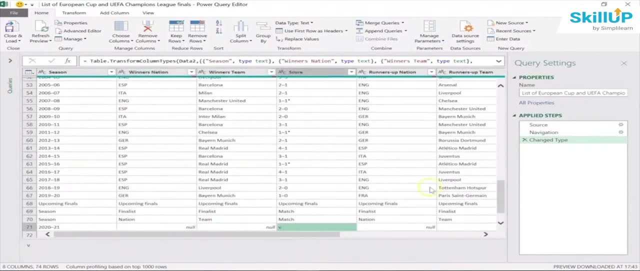 some rows which have null values. so actually these rows do not add up any value, or do not add any value to our data. so we'll clean this data first. so let's see how to do it. if you want to remove certain rows in the table, you need to remove certain rows first and then remove certain rows in the table. 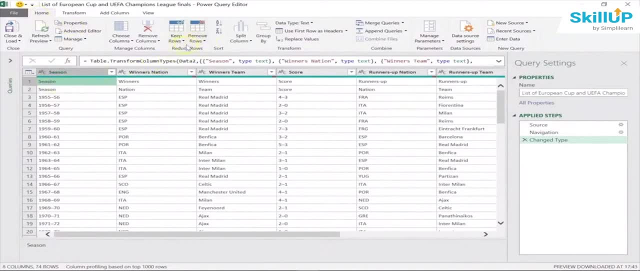 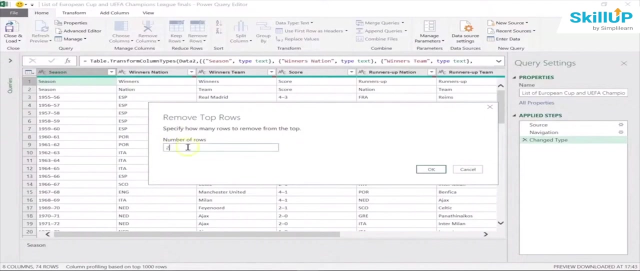 what you can do is go to the home tab and, under reduce rows, click on remove rows and then choose remove top rows. if i select remove top rows, it will ask me: how many rows do you want to remove from the top? you can see it here. i'll give: i want to remove the top two rows. now let's click on okay. 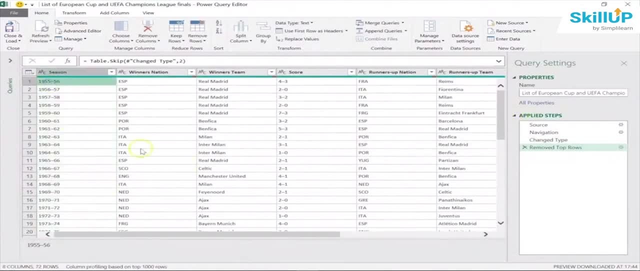 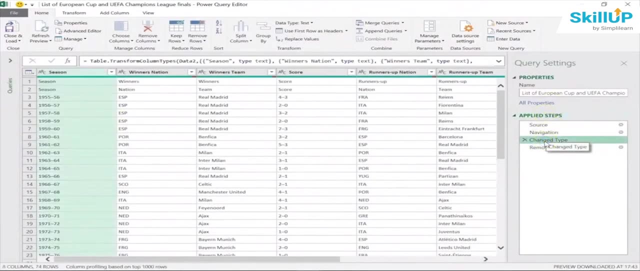 you will see that the excel power query editor has removed the first two rows and on the right you can see the steps that were applied. you can see it here: previously we had these two rows which were redundant, and once we applied this step, it has removed the first two rows. similarly, let's go. 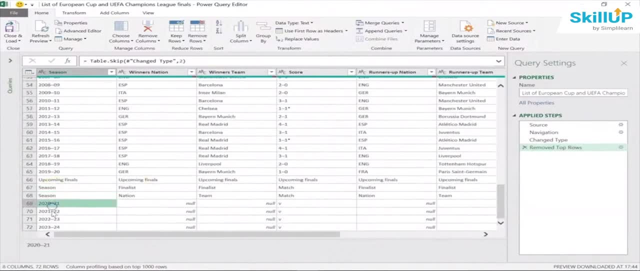 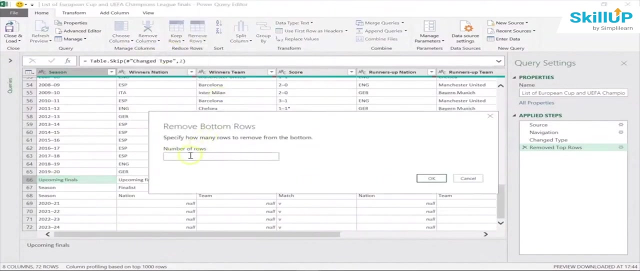 down and remove the last one, two, three, four, five. so we are going to remove the last seven rows from the table. so again, i'll go to reduce rows and click on remove rows now. this time i'll select remove bottom rows and here i'll choose. i want to delete seven rows from the table, from the bottom. i click on okay, if you see. 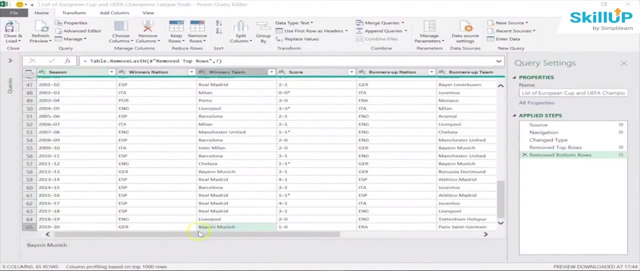 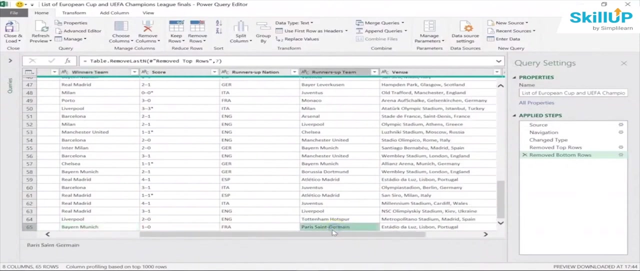 the last seven rows have been deleted. let me show you the last row, which is this one. so the last season of ufa champions league was held in 2020, which is this year, and bayern munich won the champions league against a french team, that was paris saint germans, by a score of 1-0. 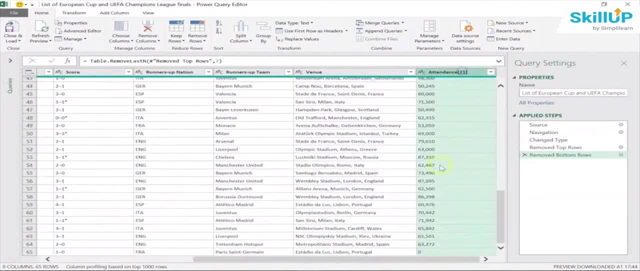 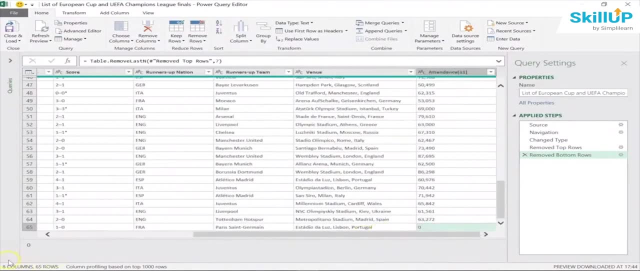 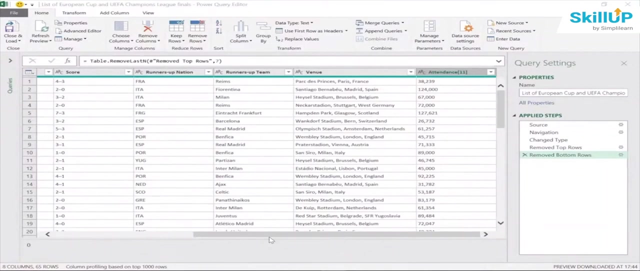 now, if you see the last value, that is, the attendance, you can see the value is 0, which means there were no spectators in the stadium. it was because of the covet conditions. now let's do some more manipulation to our data, suppose this time. i want to add a new column, let's say a stadium name, by extracting values. 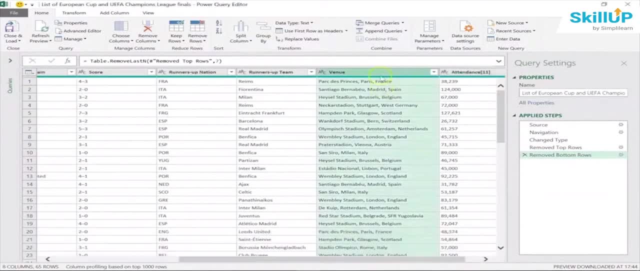 from the venue column. so let me just show you the venue column. so this is our venue column. so the first value is the stadium name, then we have the city in which the stadium is there and finally we have the country name. so i want to extract only the stadium name so you can see we have some stadiums like santiago. 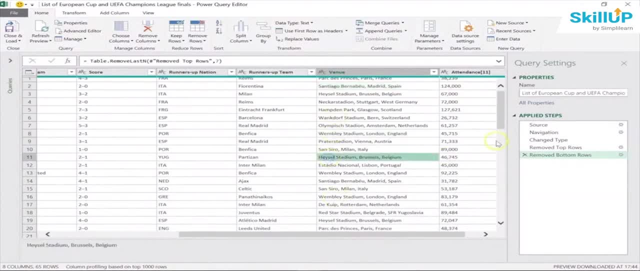 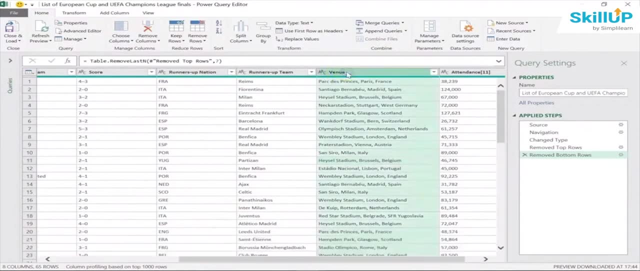 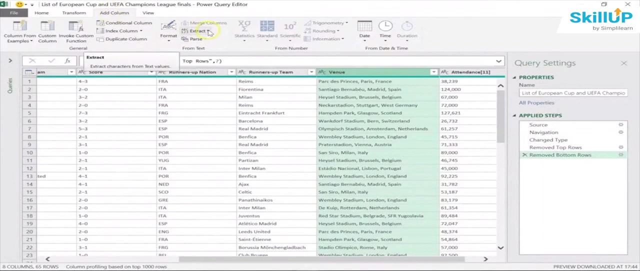 bernabeu, there's wembley, san siro and other stadiums. so i want to extract only the stadium names. so let's see how to do that. i'll click on the venue column and go to add column tab under add column. here you can see we have extract. if i click on this drop down there's an option to. 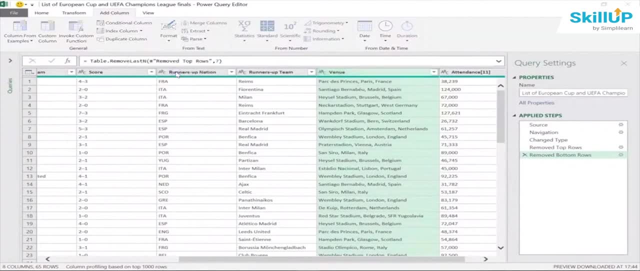 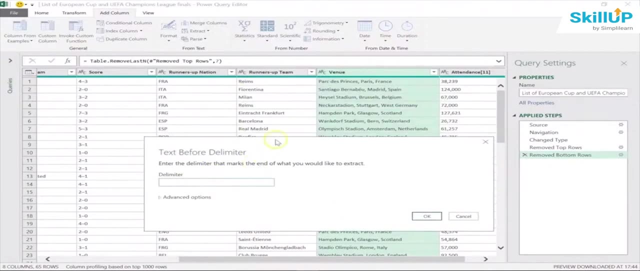 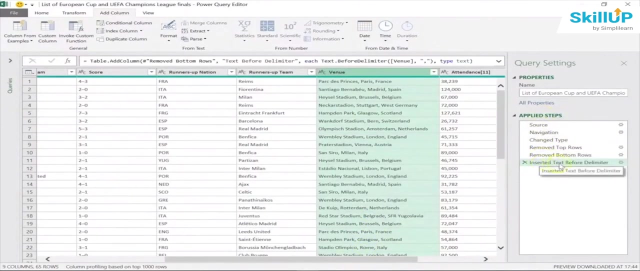 select text before delimiter. so if i choose text before delimiter here i'll give my delimiter as comma. so everything before the first comma will be considered as the stadium name. now let me click on ok. now here you can see under applied steps it says inserted text before delimiter. if i scroll 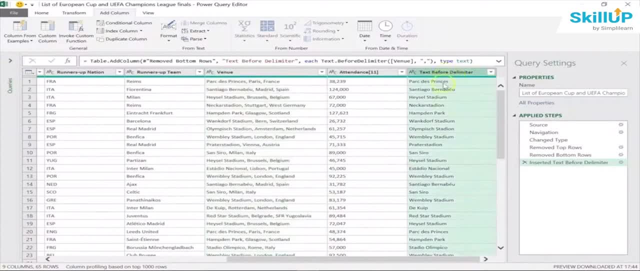 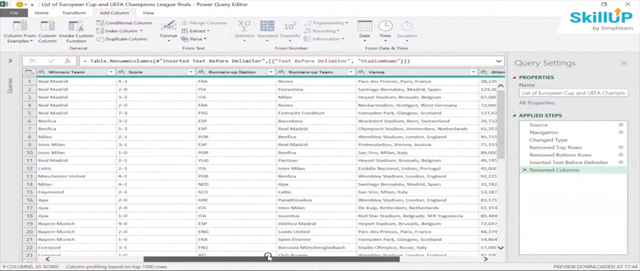 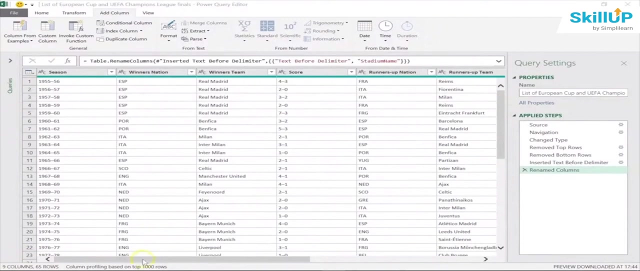 to the right. you can see the last column has our stadium names. let me double click on this and change this to stadium name column and hit enter. even this step is applied here. you can see renamed columns. similarly, let's explore a few more features. now i want to add a new column called stadium city. so if you consider this venue column- whatever is, 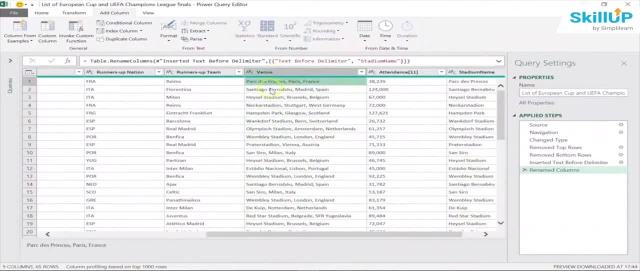 there, between the two commas, is the stadium city. so, for example, santiago bernabeu is in madrid. similarly, wembley stadium is in london, san siro is in milan. so these medial values i want to extract into a new column called as stadium city. so let's see how to do it. so i'll click on the venue column. 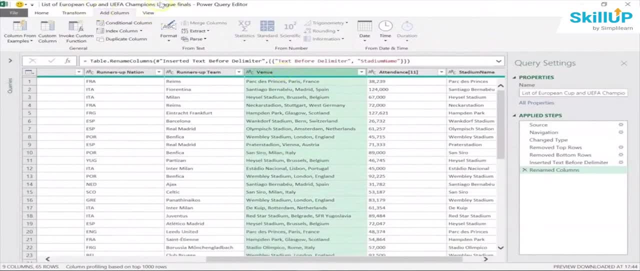 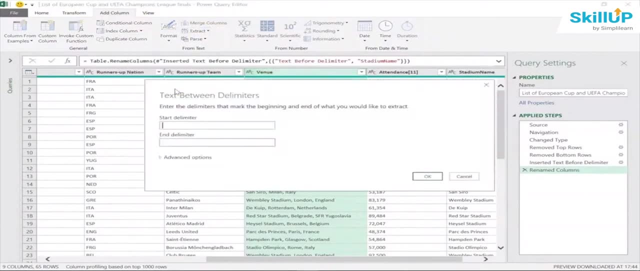 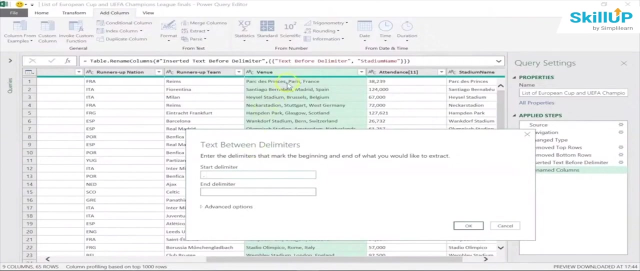 and go to extract and again i'll select the extract tab and here now i'll choose text between delimiters and my first delimiter i'll give is a comma and a space. you can see here all the values have a comma and a space and my end delimiter will be: 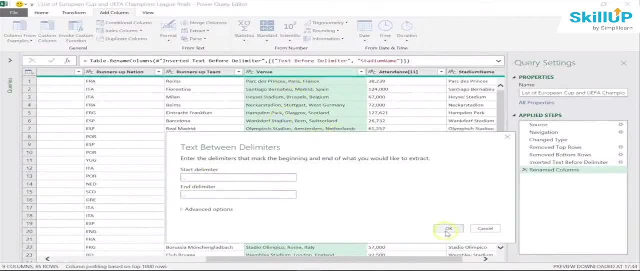 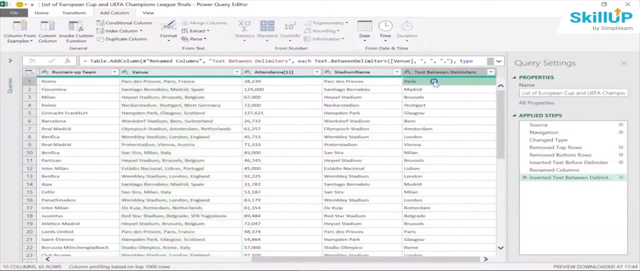 another comma, then i'll click on ok. this will add a new column to the extreme right of the table. you can see here we have text between delimiters and it has extracted the stadium city. let me go ahead and rename this column as stadium city and hit enter. you can see the applied step here. 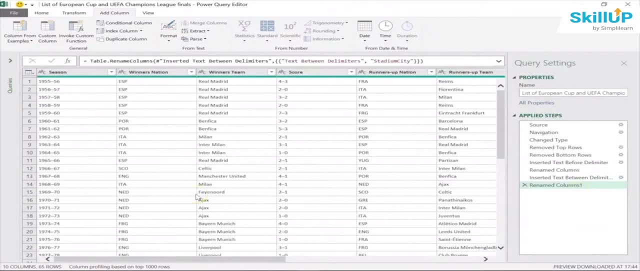 now i want to split the score column into two columns. so here we have the score column and the left value presents the number of goals that was scored by the winning team and the right value presents the number of goals that were scored by the losing team. so here i'll split the column into. 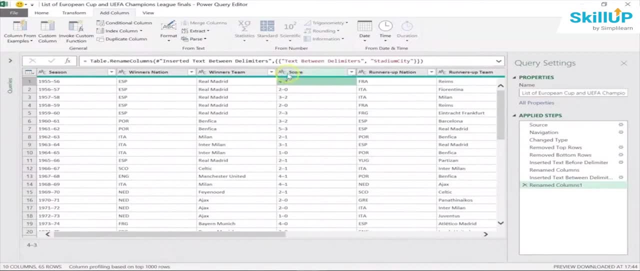 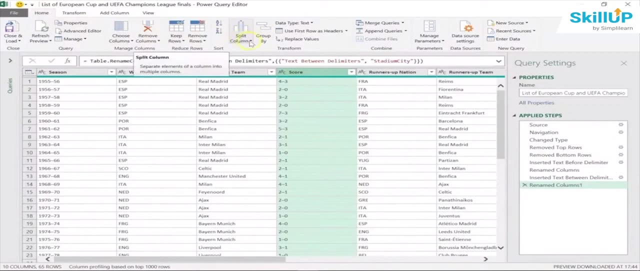 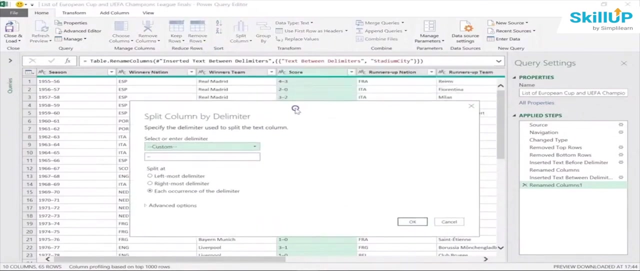 two columns as winner score and loser score. so what i'll do is select this column and go to the home tab. under the home tab we have split column. i'll select split column and then choose by delimiter. so automatically, excel power query detects that this dash is my delimiter and i'll split at each occurrence of the delimiter. let's click on ok. 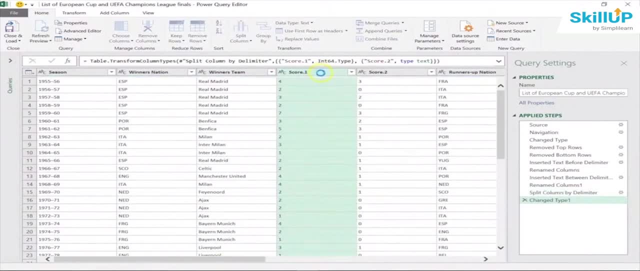 now you can see the score column has been split into two. it has renamed the column as score.1 and score.2. what i'll do is i'll go ahead and we'll rename this column as winner score and this will rename it to loser score. i'll hit enter and i have. 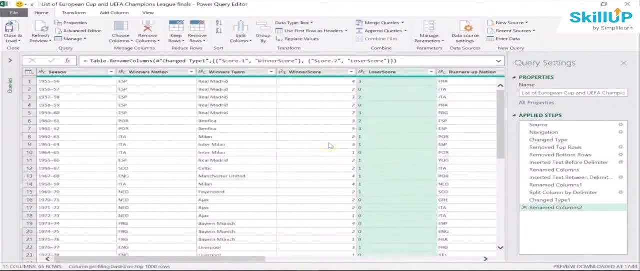 renamed it successfully. next, let's change the winners team and the runners up team values to uppercase. so suppose i want to change all the values or the club names of the winners team to uppercase. so what i can do is i'll select this column and go to the transform tab under transform. 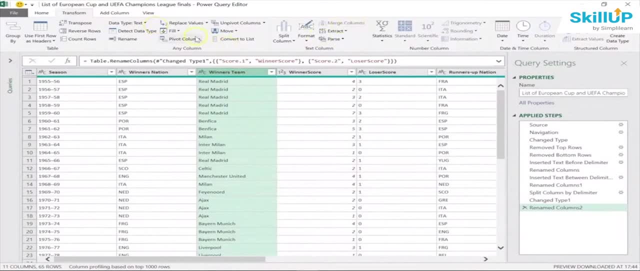 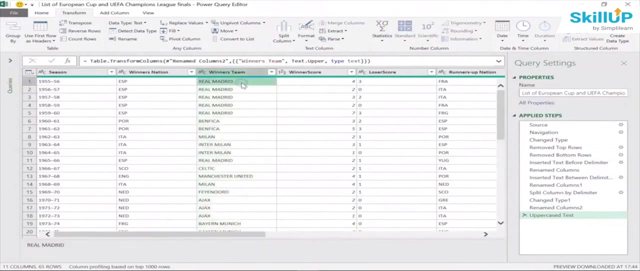 tab i have this option called format. so here i'll click on format and then you can see i can change the case to lowercase, uppercase, capitalize each word. so here i want to make all the winner teams as uppercase. i'll select uppercase. there you go. we have successfully converted all the winner team. 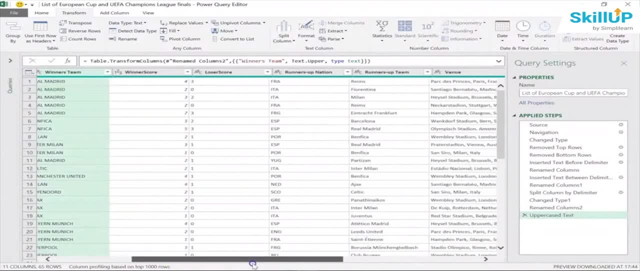 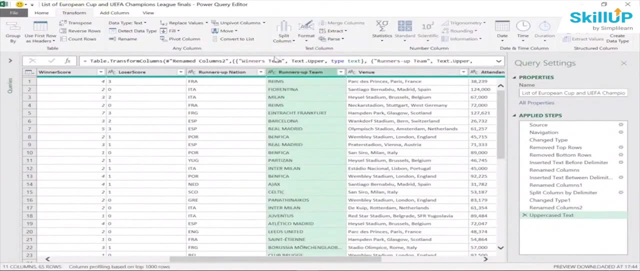 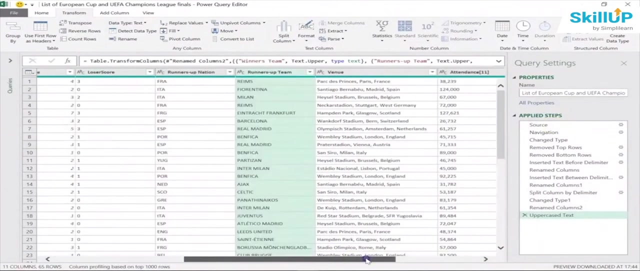 names to uppercase. similarly, let's do it for the runner sub team as well. so here i have my runner sub team. i'll go to the transform tab, click on format and select uppercase. now we saw how to do some simple manipulation of our data, so we created a few columns, split a few columns now to save all. 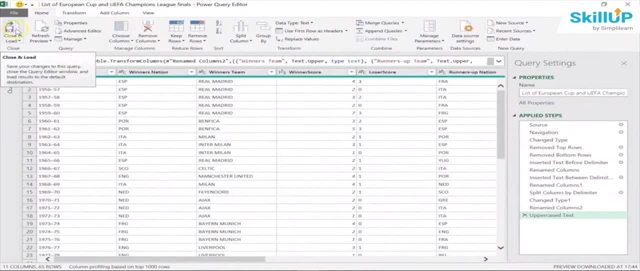 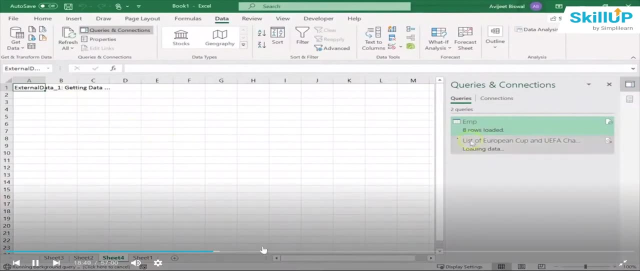 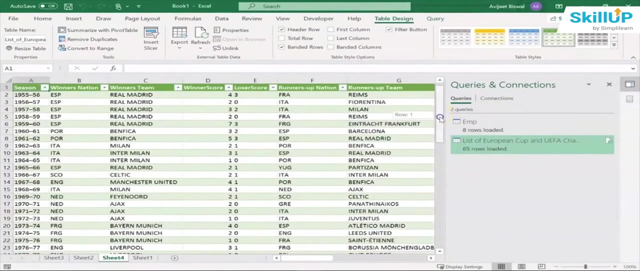 this. i have to go to the home tab and then click on close and load- this will take some time- and load our data onto this excel sheet. you can see here it's loading the data. this will take a bit of time. there you go. excel power query feature has successfully performed some manipulations. 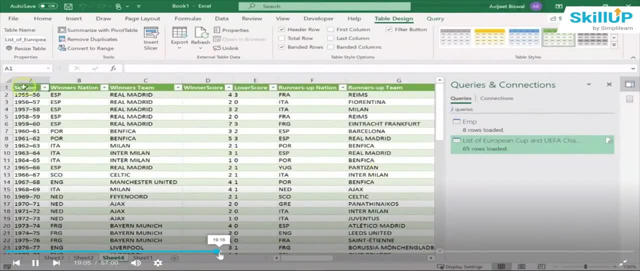 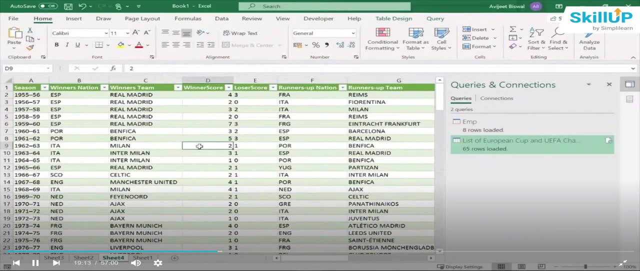 on our data, some calculations on our data, and then it has saved the final version and loaded it onto excel. now, using this clean data, we can do some analysis. let's say, i want to find the seasons in which the winners team scored more than three goals. so we have a problem statement at hand. we want to find the seasons in which the winner team 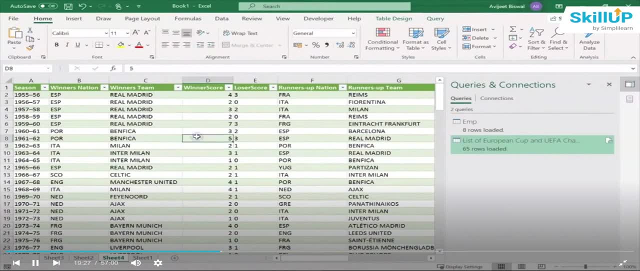 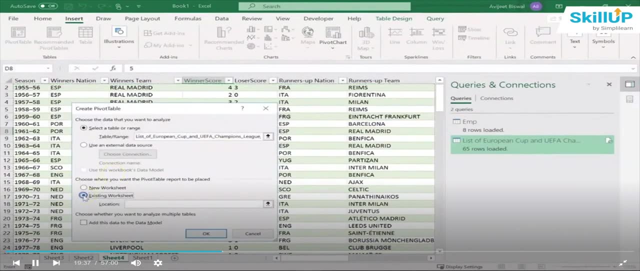 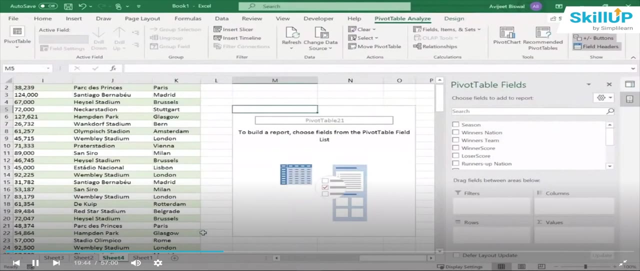 had more than three goals scored. so what you can do is select any cell in this data and go to the insert tab and click on pivot table. here i'll click on existing worksheet and then i'll give my location. i'll please my pivot table somewhere here and click on ok, all right now, since i want to know the seasons. 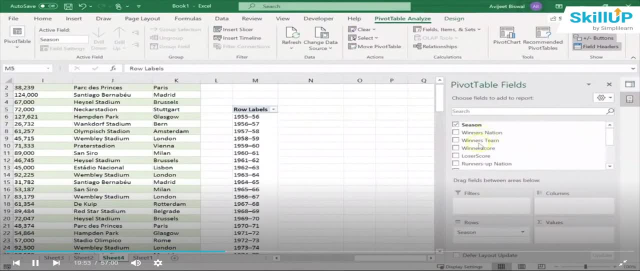 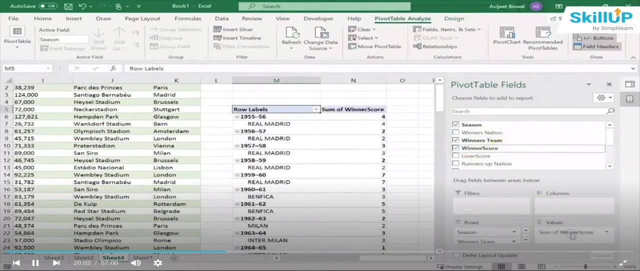 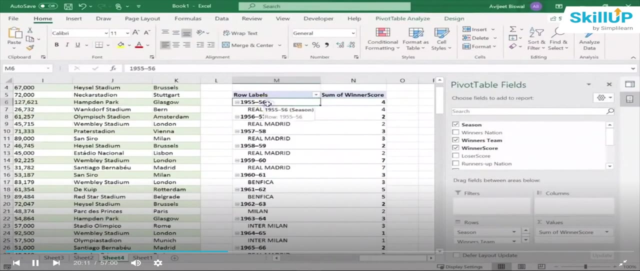 i'll drag season on to row and i'll also drag the winners team column on to those. then i'll choose my winner score under values. here you can see we have the pivot table ready. now we need to filter this table to see all the winning teams that scored more than three goals. 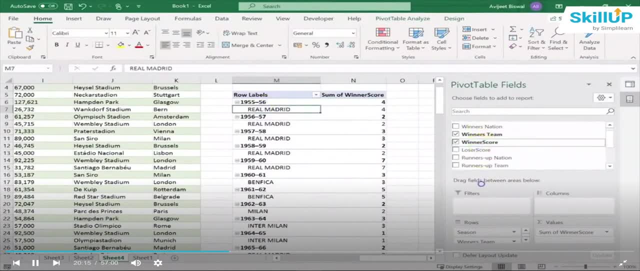 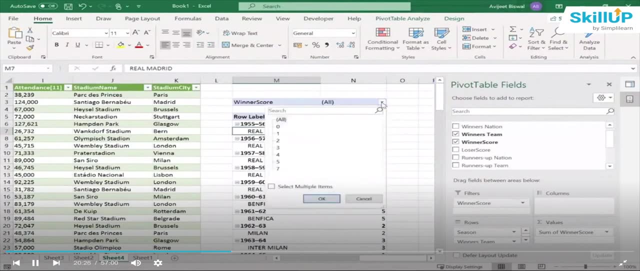 so what i'll do is i'll select this winner score column and place it on the winning team column and under filters- and here you can see i have my filter- let me click on this drop down and i'll select multiple items. from this. multiple items, i'll choose four, five and seven, because these 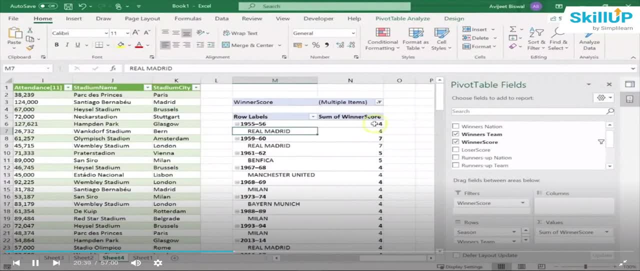 values are greater than three and click on okay. here you can see i have filtered my table and to the left you can see the season and the winner team that had scored more than three goals in the finals. all right, similarly, you can perform some work analysis, suppose. i want to know how many. 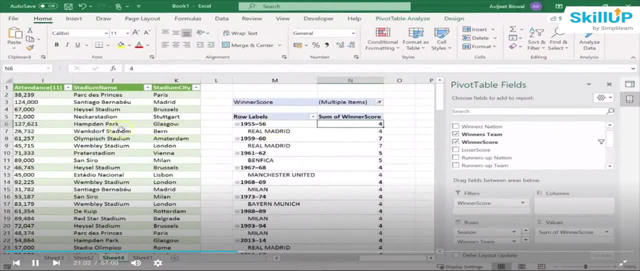 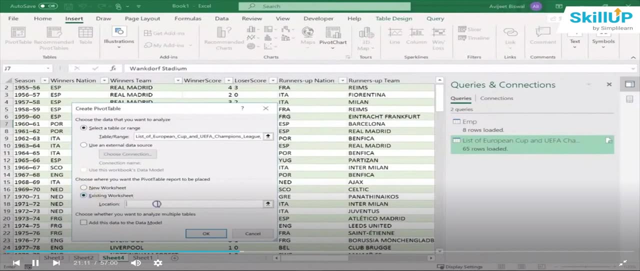 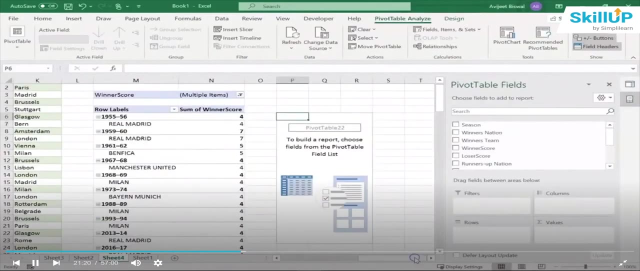 times real madrid won the championship. so let's see, i'll click on one cell in the data set, go to the insert tab and click on pivot table. i'll choose existing worksheet and give my location here. let's say, i want to place my pivot table here. click on. okay, all right. so the question we have. 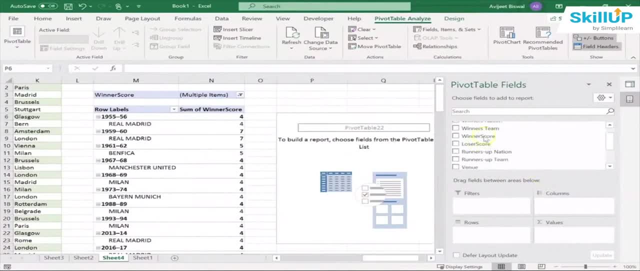 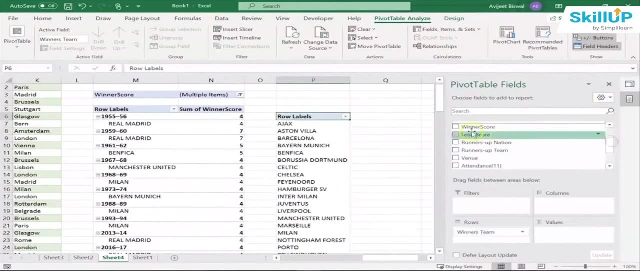 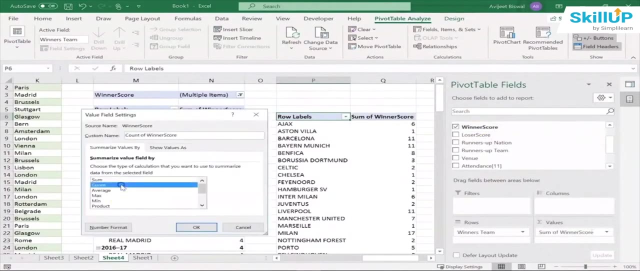 is: how many times have real madrid won the championship? so i'll choose you the winners team column and place it under rows and let's say, we'll select the winner score as well, and let's convert this winner score from sum to, let's say, count and click on okay. and 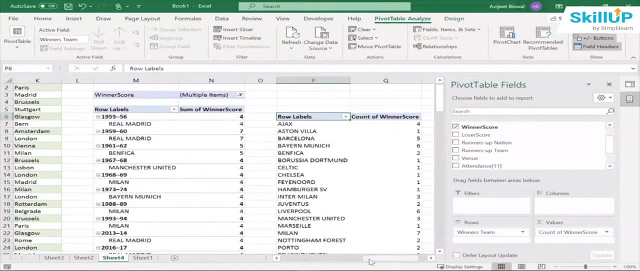 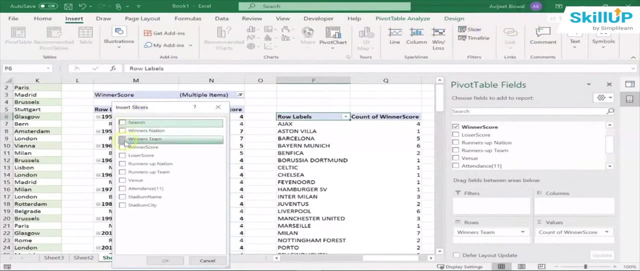 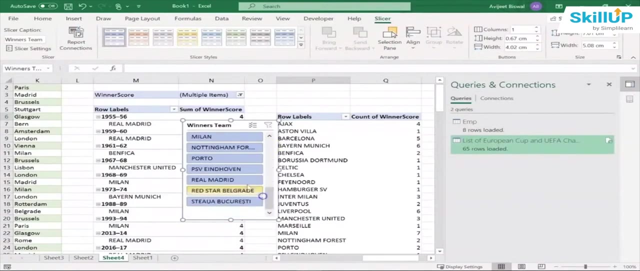 since i want to check only for real madrid. so what i'll do is i'll go to the insert tab and i'll insert a slicer here. i'll choose winner teams as my slicer and click on okay, and out of this i want to choose only real madrid, so i'll select real madrid. 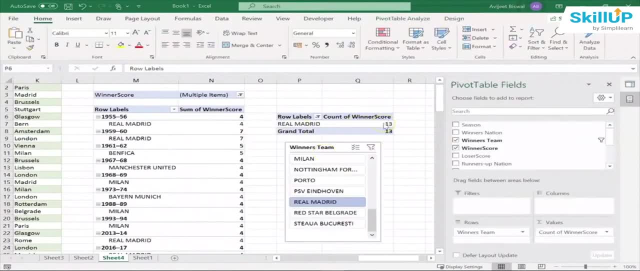 you can see it here: real madrid have won the championship 13 times. okay, let's say you want to compress your data and remove unnecessary columns without losing any information. you can do that using a feature in the power query editor called unpivot. to perform this task, we'll use a census data of india from wikipedia. so let me first show you.